So 1 plus 4 is 5, plus 2 is 7, plus 9 is 16. 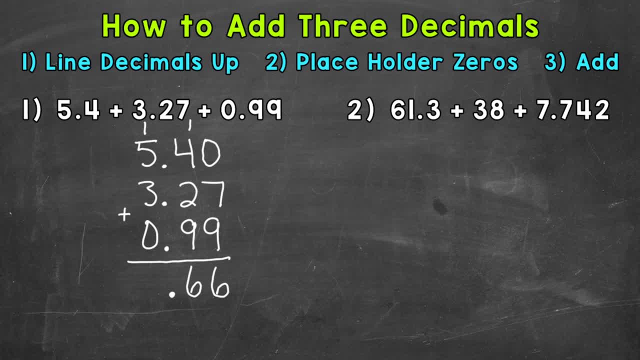 Now I'm going to bring my decimal straight down into my answer. That decimal should be lined up throughout the entire problem. Now we add the ones. So 1 plus 5 is 6, plus 3 is 9. Our final answer, 9 and 66 hundredths. 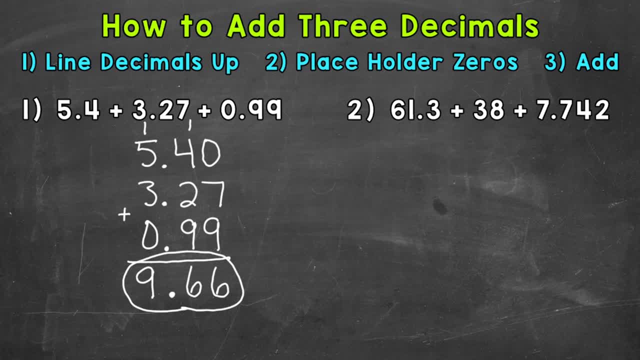 Now I do want to mention one more time where to place the decimal in the answer. So bring the decimal straight down. Decimals should be lined up throughout the entire problem when we add decimals, even in the answer. So again, bring that decimal straight down. 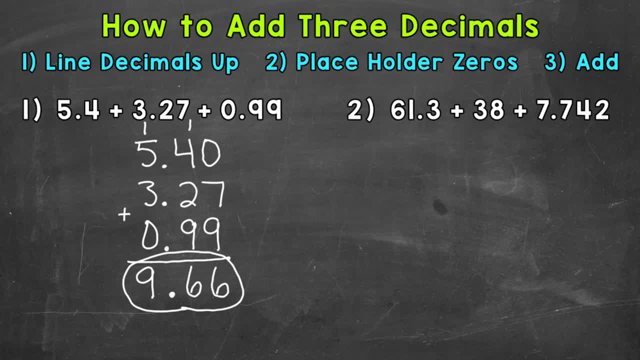 Let's move on to number 2, where we have 61 and 3 tenths, plus 38, plus 7 and 742 thousandths. Let's line this problem up. So 61 and 3 tenths, plus 38. 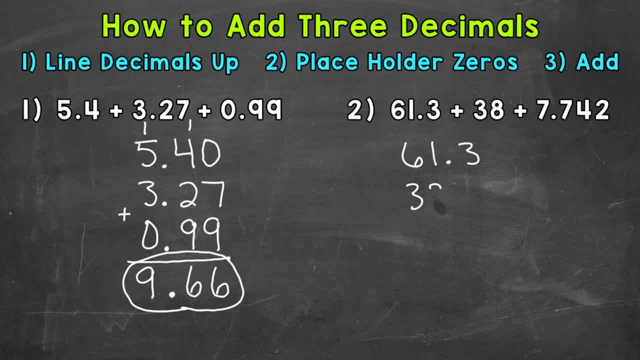 Now 38 is a whole number, but it still has a decimal. Whenever you're working with a whole number and you need to line up decimals, decimals come after whole numbers. 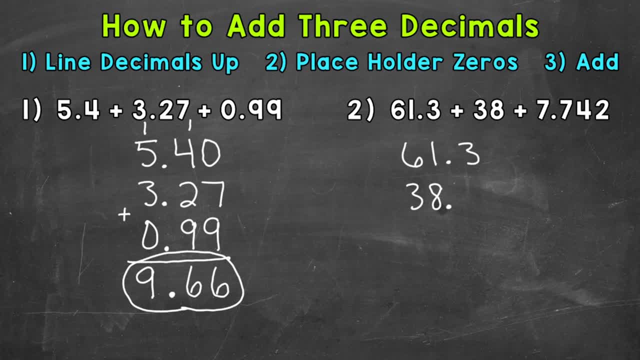 So the decimal comes after the 38. Then we have 7 and 742 thousandths. So let's use some placeholder zeros to get this problem. Lined up a little better. So everything needs to go to the thousandths place. And now we're lined up and ready to add. So start with the thousandths. We have 0 plus 0 plus 2. That's going to give us 2. 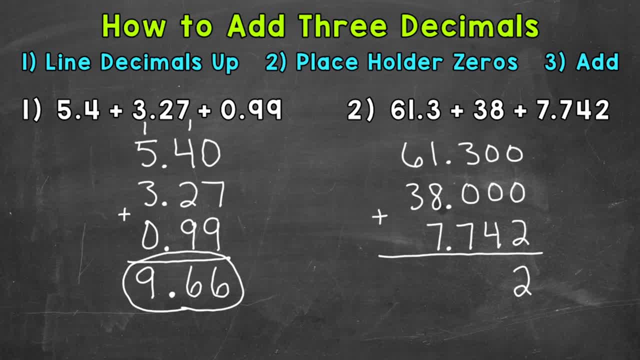 Now for the hundredths. 0 plus 0 plus 4. That gives us 4. Now the tenths. 3 plus 0 plus 7. That gives us 10. So we put our 0 and regroup or carry the 1. Bring our decimal straight down. And now we add the ones.